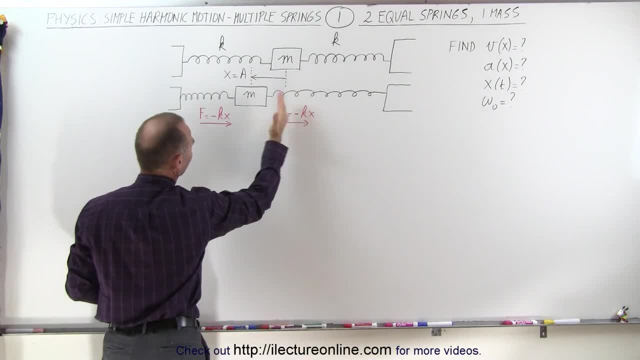 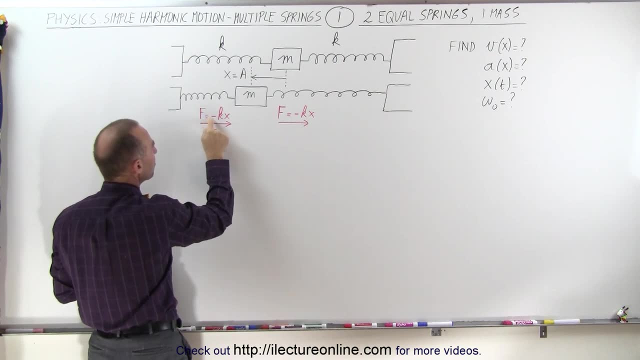 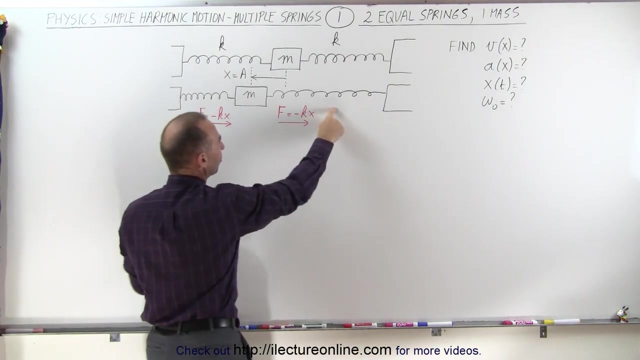 equilibrium point. Notice, when we push the object to the left a certain distance, this spring will be compressed and we'll be pushing to the right. Notice, with Hooke's law we have f equals minus kx, but since x is a negative value, that will then be a force in the positive direction This spring. 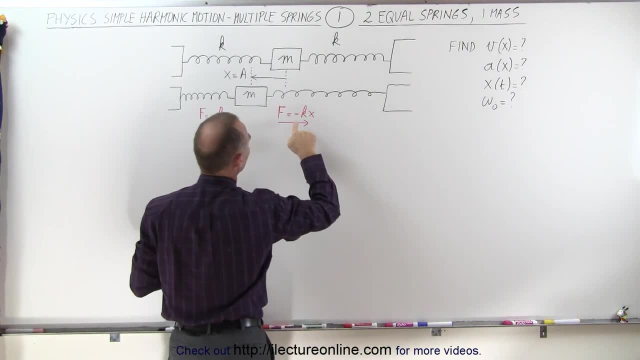 will, of course, pull in this direction because you're elongating it. but again, f equals minus kx and since x is a negative quantity, when you move to the left- negative times, negative is positive- you can see that both springs will be pushing and pulling on the object in this direction. 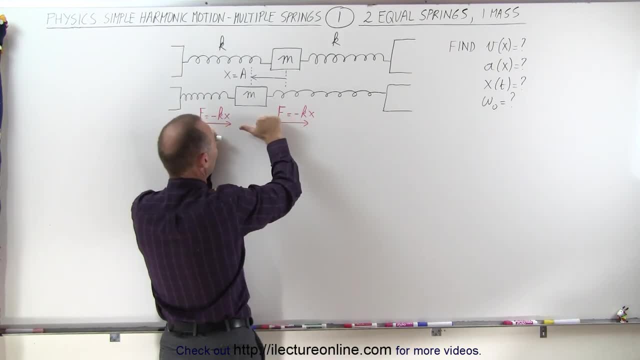 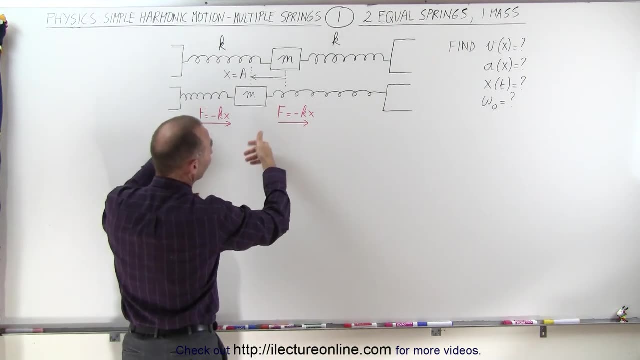 or when the object is pushed in this direction, both forces will be in the negative direction, But you can see that both springs will act in unison and pushing and pulling in the same direction, that no matter which side of the equilibrium point the object is at. 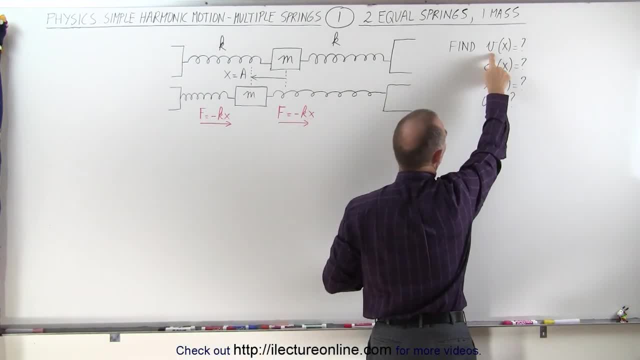 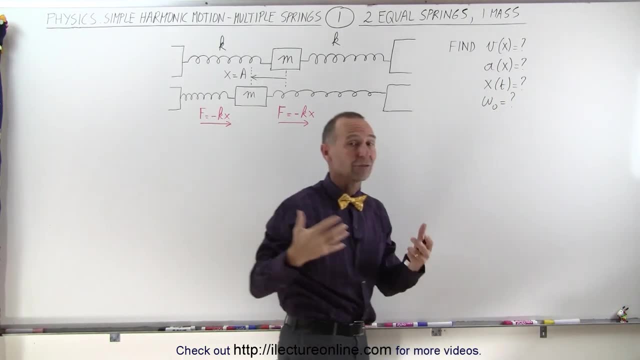 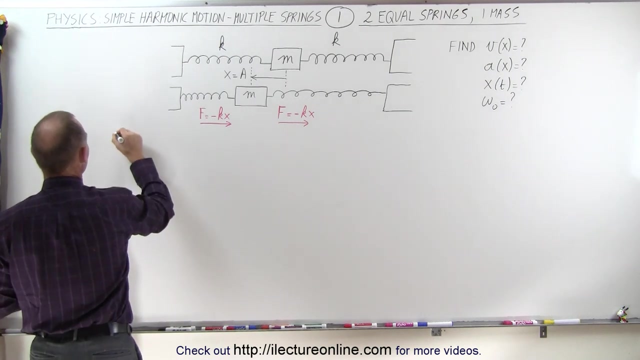 What we're trying to find is: we're trying to find the velocity as a function of position. the acceleration is the function of position, the position is the function of time, and we're trying to find the natural frequency of this particular setup. the way to do that is to start out by saying that the total energy that's contained in the system is equal. 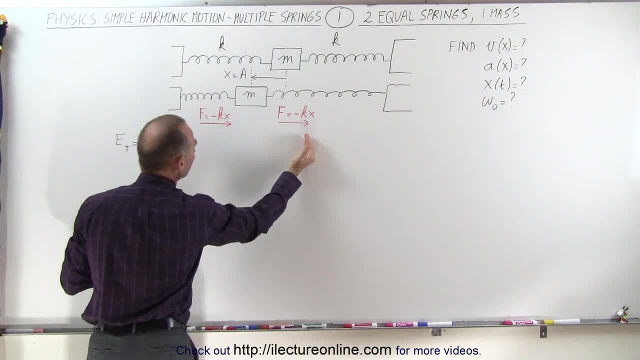 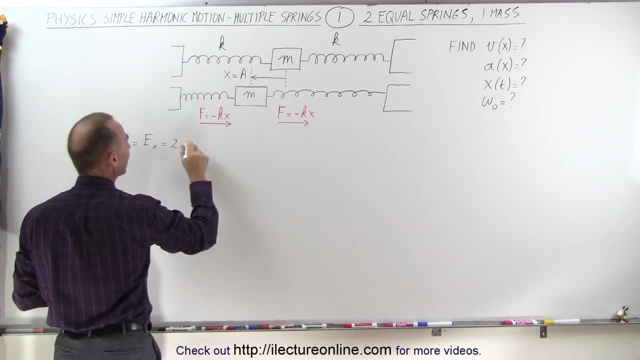 to the initial energy that we put in the system when we take the block and move the maximum distance a away from the equilibrium point. that means that at that point we have twice the energy stored in the spring because we have two springs with the same spring constant. so it's two times. 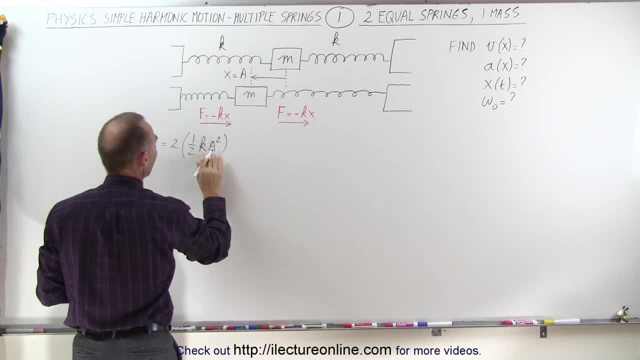 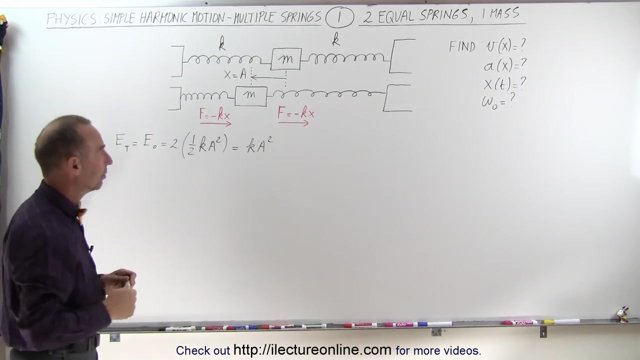 one half k a squared, because x will be the maximum displacement. so this will be k a squared as being the maximum energy put into whole system. now, once you let go and the system starts oscillating back and forth, then the energy will be divided in different proportions in both. 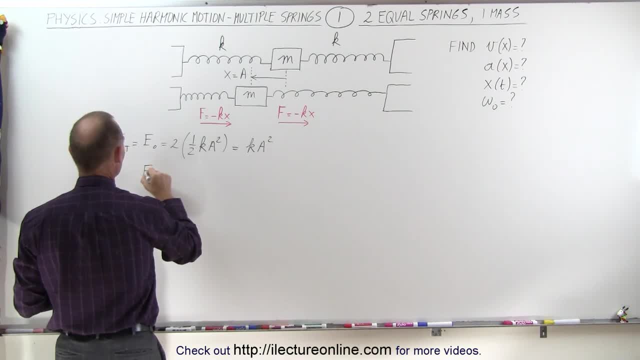 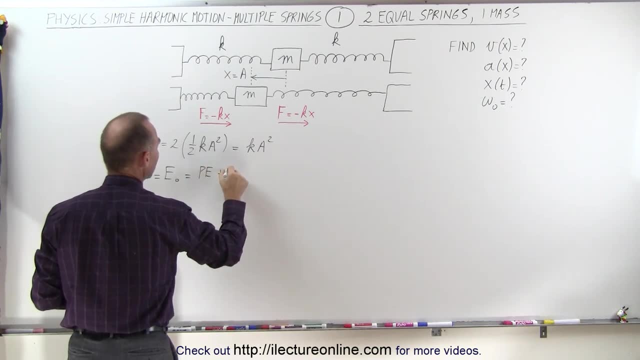 kinetic and potential energy. so then the energy, which is still always going to be equal to the energy that we put in the system, is equal to the energy that we put in the system to the initial energy, is going to be equal to the sum of the potential energy plus the kinetic. 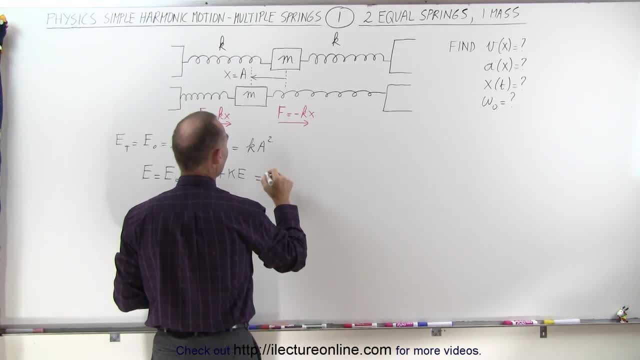 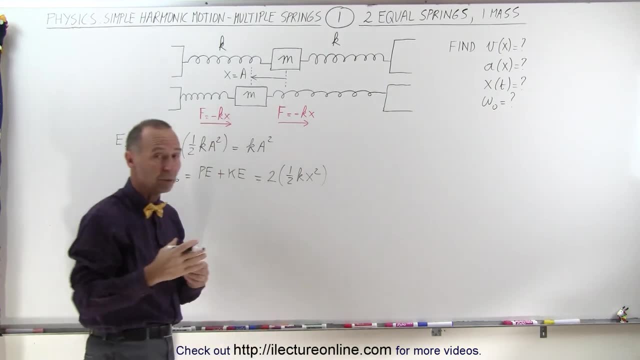 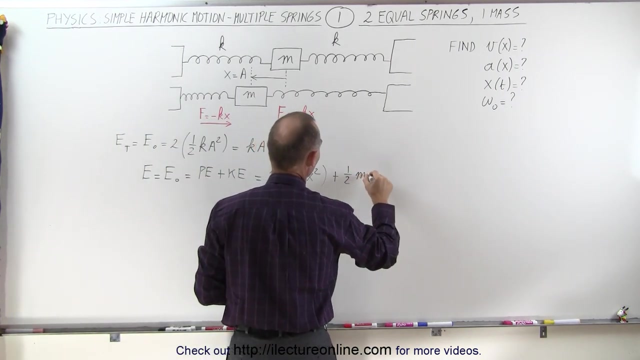 energy. so the potential energy would be equal to- and there's two springs, so it'd be two times one half k x squared, x being somewhere between zero and a or zero negative a for the springs, plus one half m v squared, and of course that then always equals the initial energy, which is equal to. 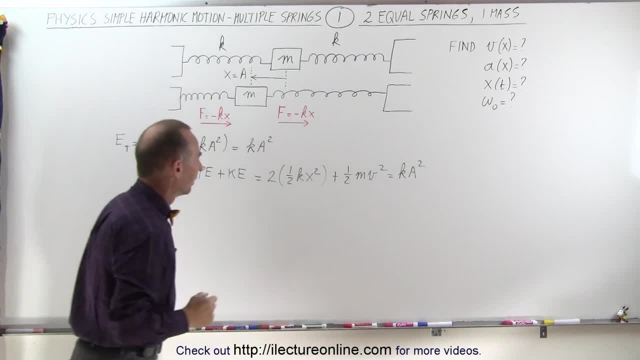 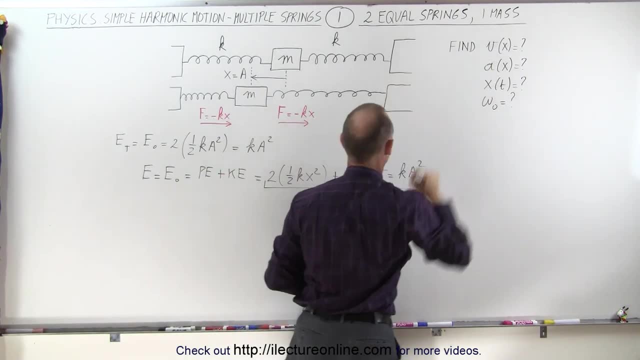 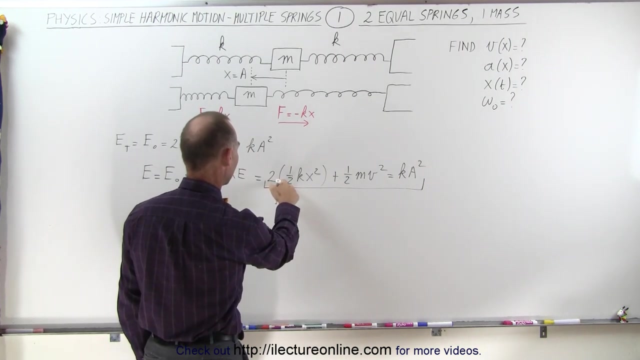 k a squared. we can then take this part of the equation and we're going to solve this for v as a function of x. so we're going to solve this for v and notice we can first multiply everything. well, let's see here: this times this gives us k x squared. if i multiply everything by two, i get 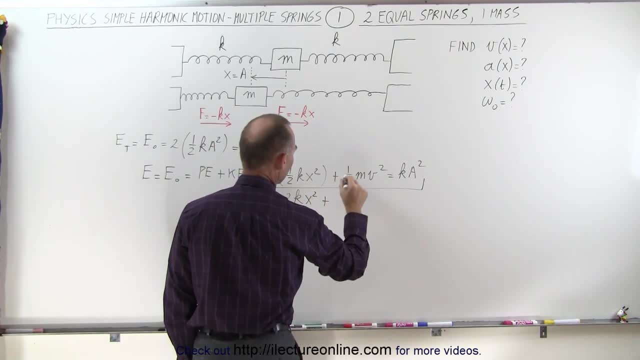 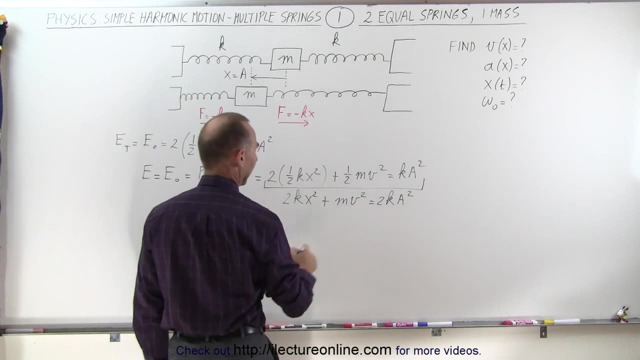 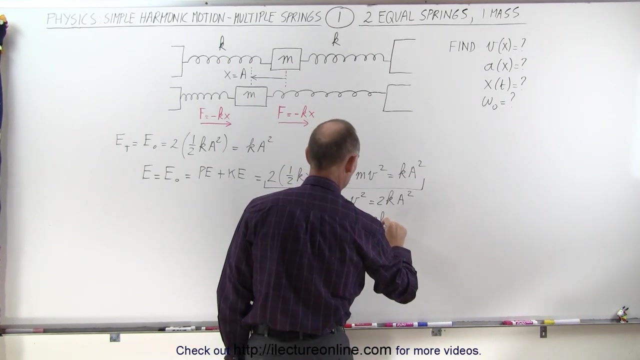 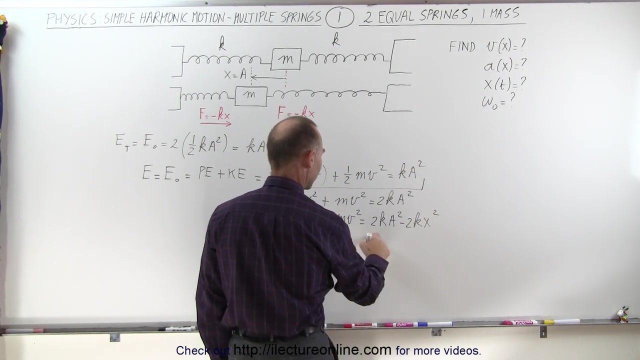 two k x squared plus two times one half is m v squared equals two k a squared. and then moving this to the other side and then we can have: m v squared is equal to two k a squared minus two k x squared. and pulling out a two k and dividing both sides by m, 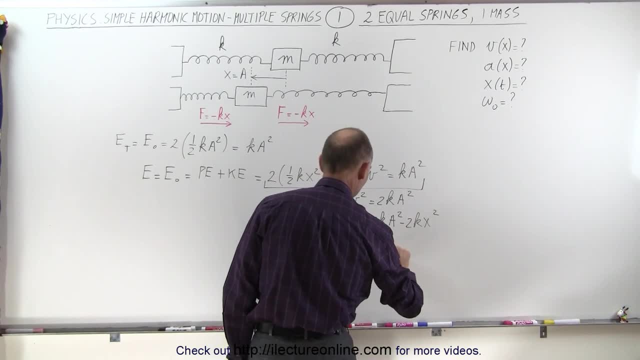 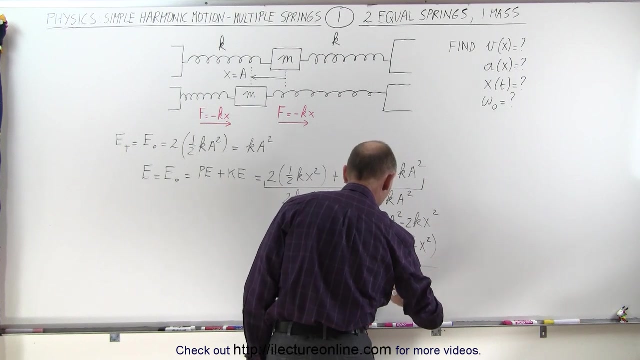 we get: v squared is equal to two k over m times a squared, minus x squared. and finally, of course, if i take the square root of both sides, i get v, which is, as a function of x, is equal to the square root of 2 k over m times a squared, minus x squared. 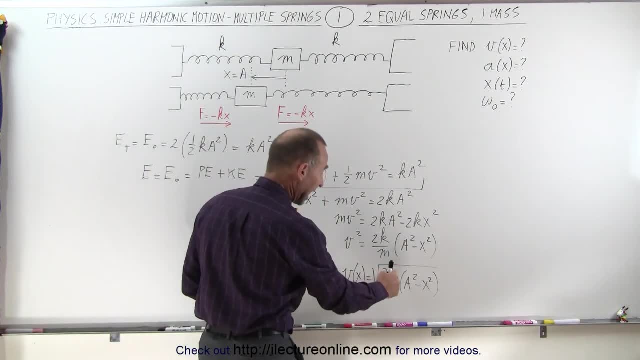 now, normally, if i have only one spring, this would be the square root of k over m times a squared minus x squared. but since we have two of them and they both work in tandem, then you can say it's 2 k over m. this then becomes the natural frequency of the system. 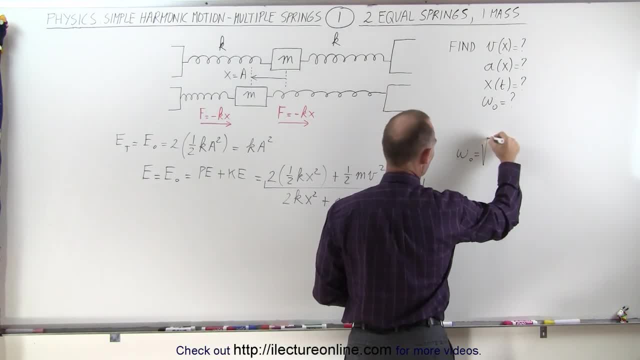 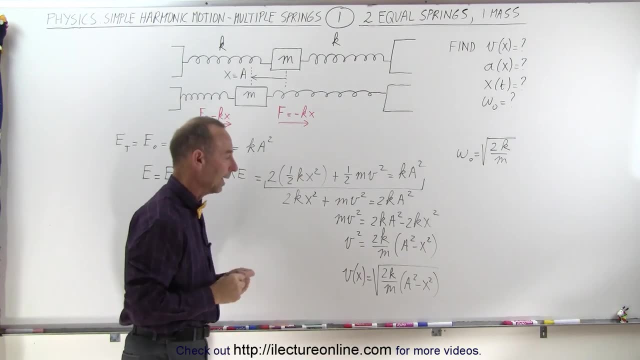 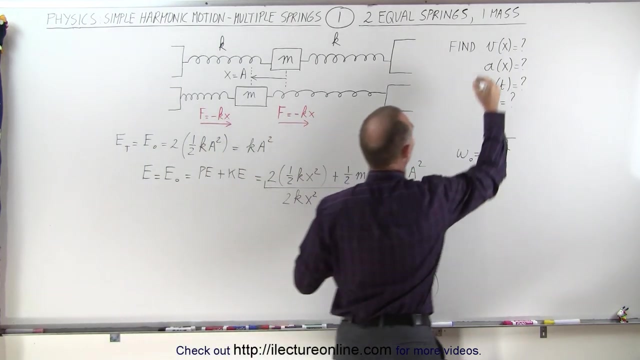 in other words, omega sub naught is equal to the square root of 2 k over m, instead of just k over m for a single spring system like that. now we still want to find the acceleration as a function of position. so we now have the velocity of the function position, we have the natural frequency of the system. 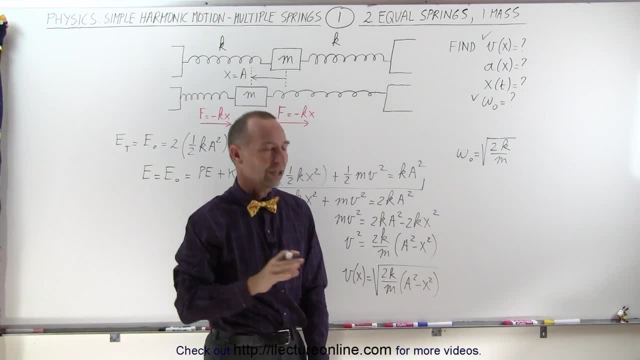 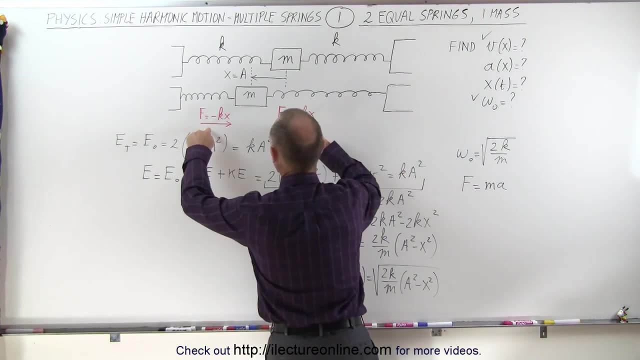 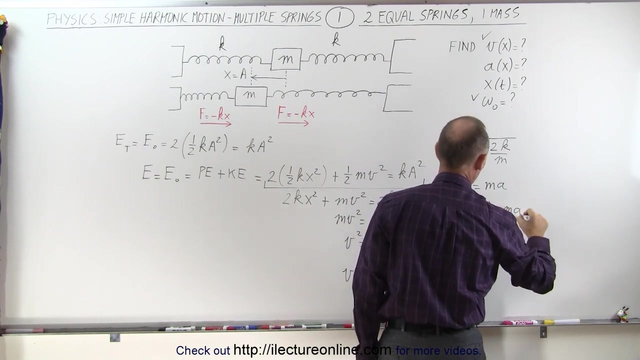 now we're going to find the acceleration for that. we use newton's second law. we can say that f equals m? a and of course, the force acting on the system is going to be the force of both of these springs. it's going to be two times minus kx equals m, a or a as a function of x is equal to minus 2 k over m.